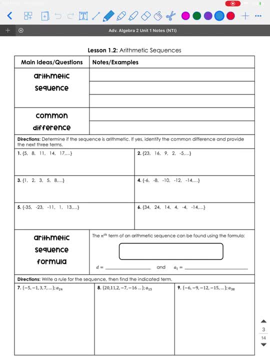 All right, lesson 1.2. I'm going to jump right in and keep this as short as possible. This is a longer lesson, so you may be looking at 20 to 25 minutes. If at any time you just need a break, that's why you have a video. You can pause it, get up, do jumping jacks, get you a snack, come back, and do all of that. This is all that you have assigned for today if you're staying on pace with me. So, you know, 20 to 25 minutes. I get it. It's not the most fun thing you could do, but hopefully it won't be that hard for you. So, Yester, the last lesson we talked about sequences and what is a sequence. Well, now we're going to get into one of the two types of sequences. The first type is arithmetic sequence. Not arithmetic, arithmetic sequence. And an arithmetic sequence is a sequence. 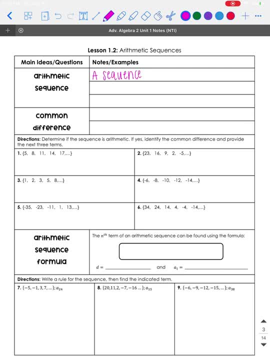 A sequence that adds by the same number each time. So, every time, if I look at all of my terms, every number in the sequence, I'm like adding, I'm doing plus three, plus three, plus three, or subtracting. If I do, if I go from like five to four to three to two to one, I'm subtracting one. That is the same thing as saying plus negative one. So, I'm still adding, but I'm adding negative one. All right, well, what is a common difference? Well, the common difference is that number that is being added. 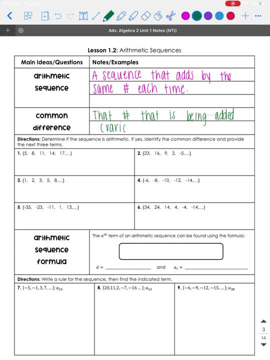 And we abbreviate that with the variable D. Oops. D for difference. 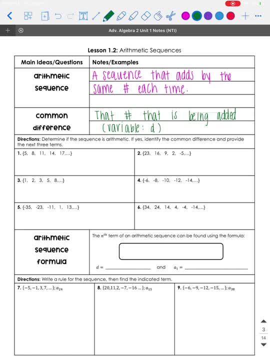 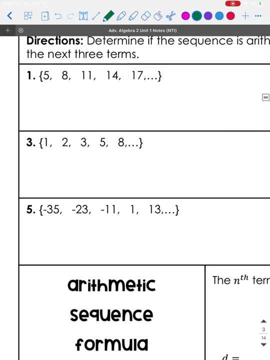 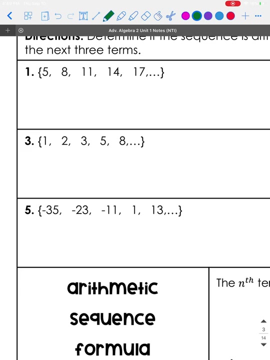 So, we're going to look at some examples where we decide if they are arithmetic, meaning they add by the same number every time and if they're arithmetic we're going to see if or what the common difference is and we're going to find the next three terms. So let's look at number one. Anytime you're checking to see if it's arithmetic you need to check all the numbers all the way through the numbers that it gives you. So if I look from five to eight. Five plus three is eight plus three is eleven. From eleven to fourteen plus three and plus three again. So since I added three every time that means that yes it is arithmetic. 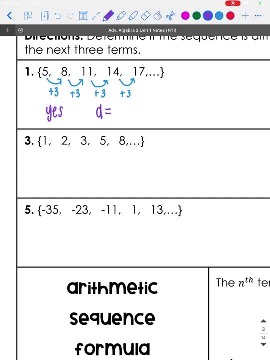 My difference is three and now we need to find the next three terms. So if I'm adding three each time I would have twenty, twenty-three and twenty-six. 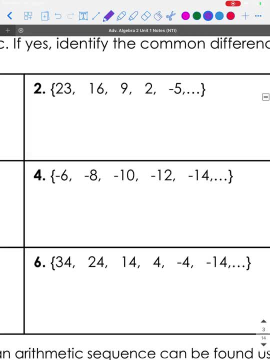 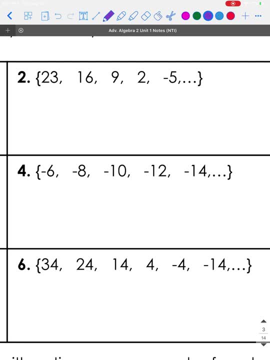 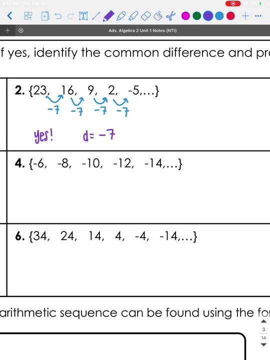 Number two. Let's look. Now my numbers are getting smaller. So that means I'm going to be adding a negative or subtracting. So from twenty-three to sixteen I'm subtracting seven. If you don't know in your calculator you can do sixteen minus twenty. Twenty-three and you get negative seven. Nine minus sixteen is negative seven. Two minus nine. Negative seven. Negative five minus two. Negative seven. So I'm going down by seven each time. So yes it is arithmetic because it goes down by the same number every time. My common difference is negative seven. And my next three terms I need to take negative five and I need to keep subtracting seven. Negative twelve. Negative nineteen. Negative twenty-six. 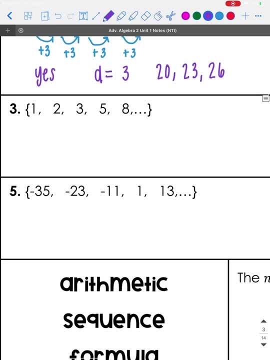 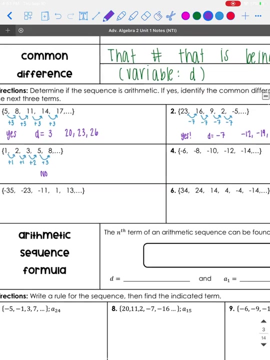 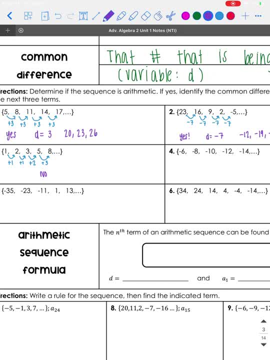 All right. Hopefully you paused the video. Now we're going to go over the answers very quickly. 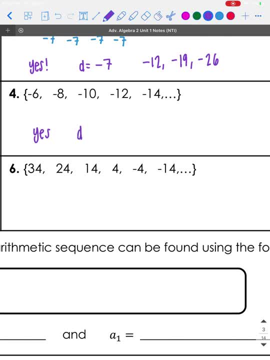 So number four is yes because I am subtracting two every time. My common difference is negative two. 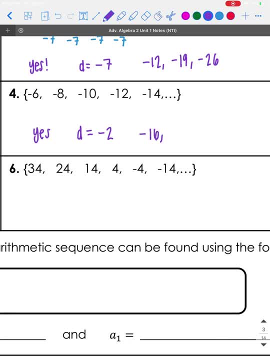 And my next three terms would be negative 16, negative 18, and negative 20. 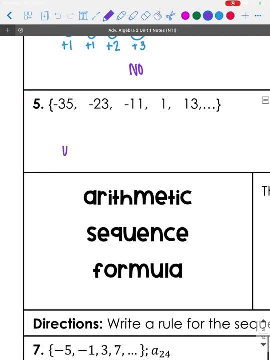 Number five is yes. My common difference is 12. I'm adding 12 each time. 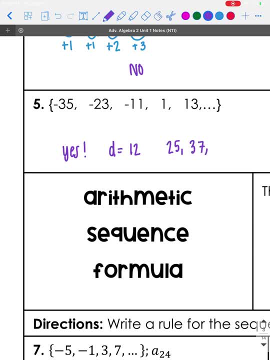 And then I would have 25, 37, and 49. 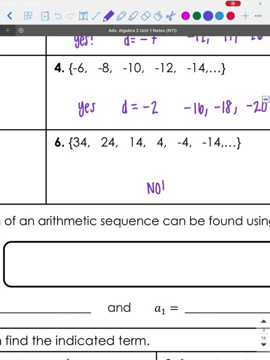 Number six. I bet I tricked some of you. The answer is no. It is not. You probably said, oh, I'm subtracting 10 every time. 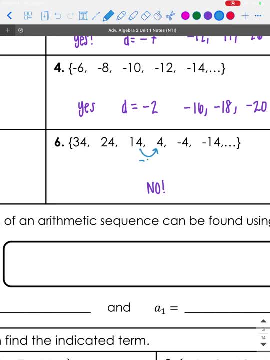 But if you look, 14 to 4, yeah, that's subtracting 10. But from 4 to negative 4, that is subtracting 8. So it is not arithmetic. 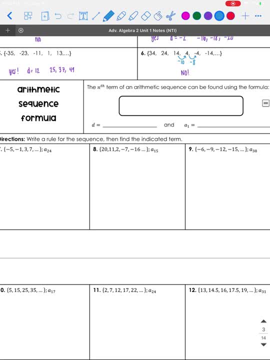 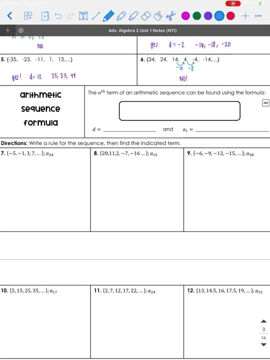 All right. Yesterday we looked at some, or not yesterday, I keep saying yesterday, but the last lesson we looked at some formulas. And you found, you learned about how to, how to find a term with the formula. Well, now I'm going to teach you how to find that exact formula. So this is the formula for an arithmetic sequence. 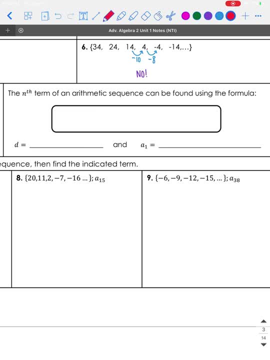 Write this in, and then I will tell you what each thing stands for. 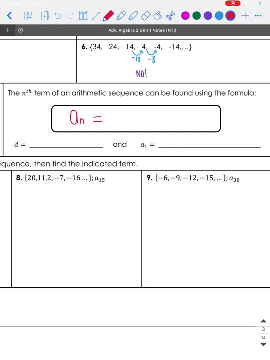 a sub n equals d times the quantity of n minus 1 plus a sub 1. 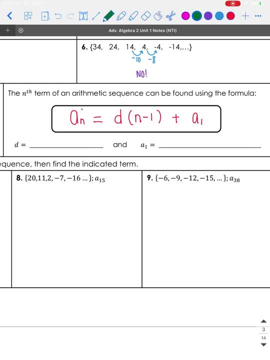 All right. So what is a sub n? Well, a sub n is just any term. So if I had the numbers 3, 6, and 7, I would have a number of n. So if I had the numbers 3, 6, and 7, I would have a number of n. So if I had the numbers 3, 6, 9, 12, 15, and so on, if I said find the 7th term, you would count in that pattern to the 7th number. 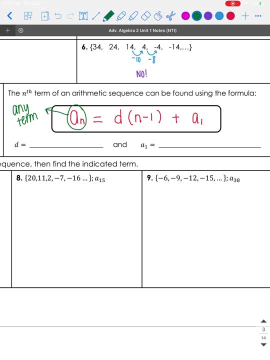 That's any term. This formula will find any term in a sequence. 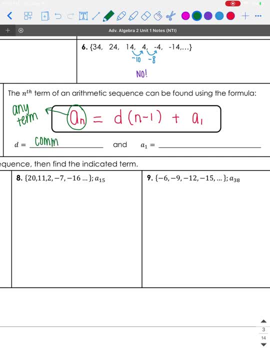 If you remember, your d is the common difference. n, that is the term number. 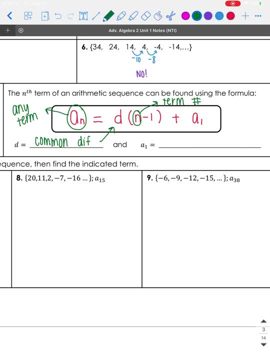 So if you were finding the 7th term, you would plug a 7 in there. 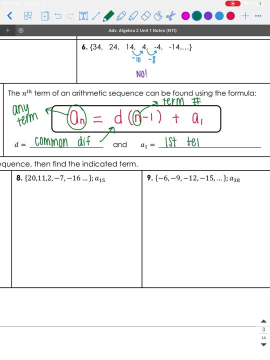 And a sub 1 is the first term. 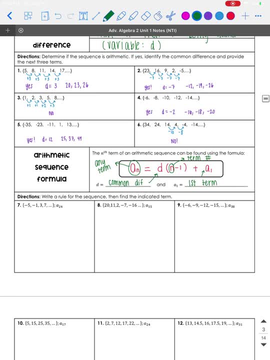 As we do some examples, hopefully this will start to make sense. It's actually pretty easy. 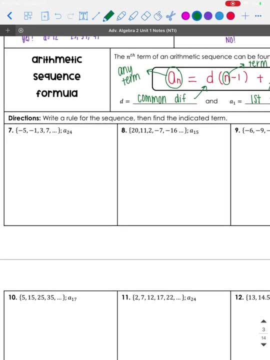 So I have some examples, and they say write a rule for the sequence. What that means is you're going to find the formula. When it says write a rule, that's the same as writing the formula. You'll just see it written both ways. So we are getting... Given the first four terms. I'm going to rewrite that formula. So I can zoom in here. 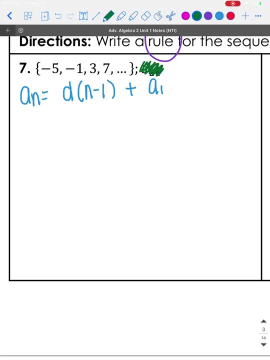 Now for the time being, I'm going to cover this up, because that's actually part 2. We don't need that yet. 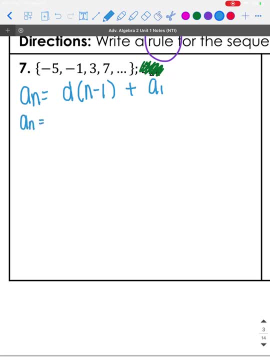 So any term. I'm going to write a generic formula that works for any term. 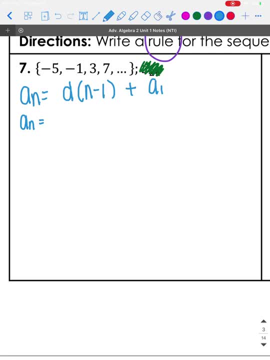 The first thing that I need is the common difference. So how am I adding, subtracting? Look at those numbers and see if you can figure out the common difference. 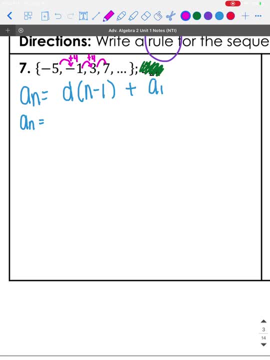 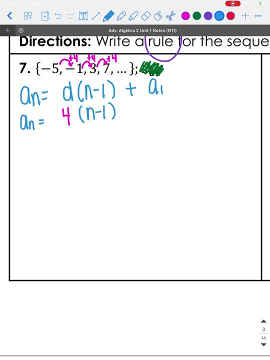 Now for now, this n minus one, you're just going to leave that. 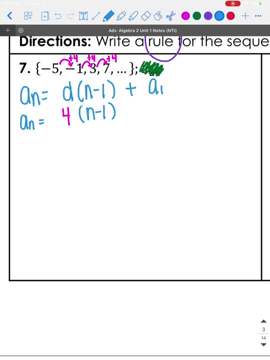 You're not actually going to plug anything in there. Because we don't... The n represents the term that we're finding. 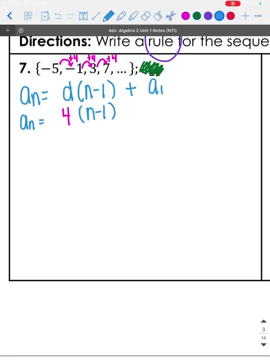 So if we're just writing a generic formula, we don't have that number yet. We don't know which one we're going to find just yet. And then I'm going to do... 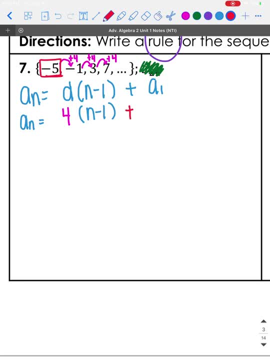 I'm going to do plus a sub one. So plus negative five. 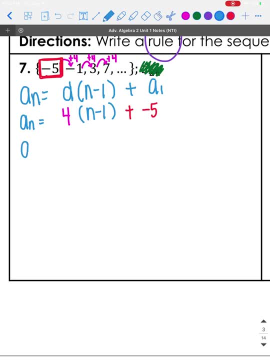 And then I'm going to simplify this. Think back to your algebra. We're going to distribute. Four times n is four n minus one. Four times negative one is negative four. And then if I have plus negative five, that's the same thing as saying minus five. 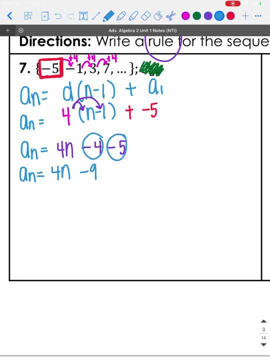 And then I combine my terms. Negative four and negative five, that's negative nine. 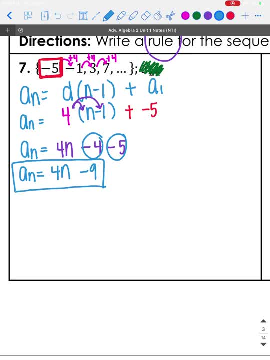 So here is my explicit formula. Or I could call that my rule. A sub n equals four n minus nine. 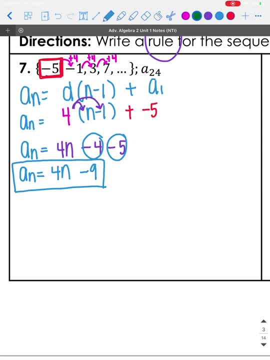 And now I'm going to find a sub 24. So I'm going to find the 24th term. 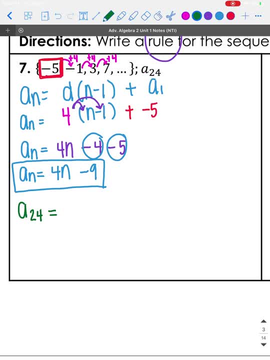 And you all did this last lesson. If you remember, we take that 24 and we plug it in for n. 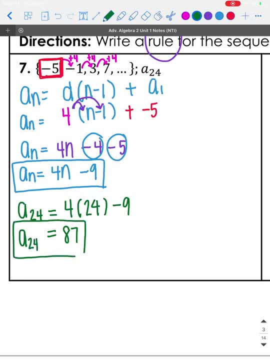 And you get a sub 24 equals 87. 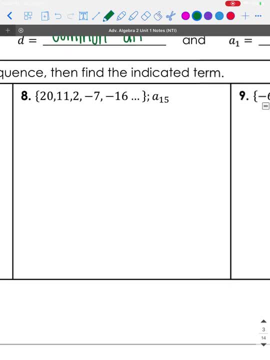 All right, let's look at number eight. We think about our formula. 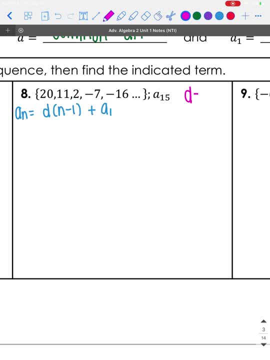 Two things that I need to know. I need to know my common difference and my first term. First term is the easy one. That's 20. 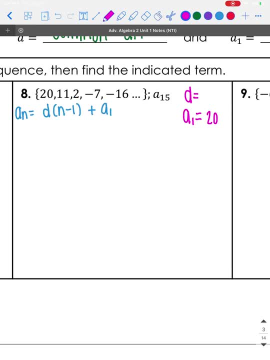 And then if I think about my common difference, how am I getting from term to term? If you don't know right off, take one, 11, and subtract the one before it. 11 minus 20 is negative nine. Test that out again. Negative 16 minus negative seven. 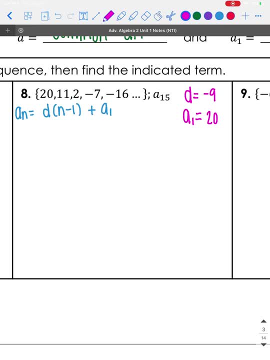 Well, that's negative nine. So my common difference is negative nine. 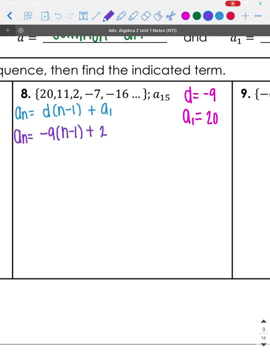 And I'm going to plug those in, negative nine. Remember, the n minus one just stays. We just keep it n minus one and plus 20. 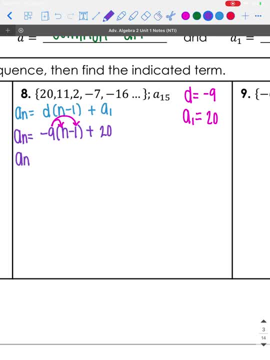 Distribute. Distribute. Distribute. Distribute. 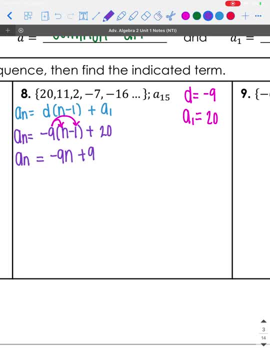 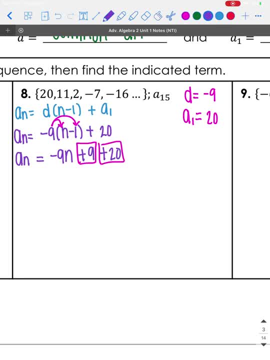 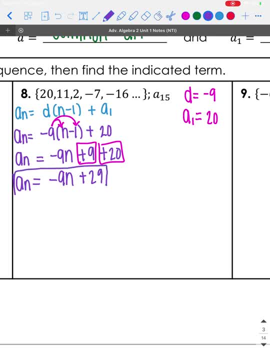 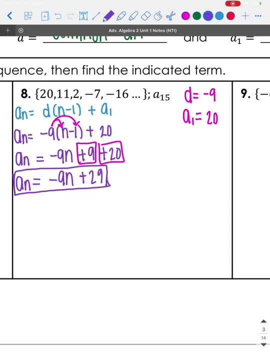 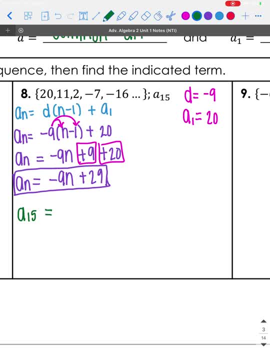 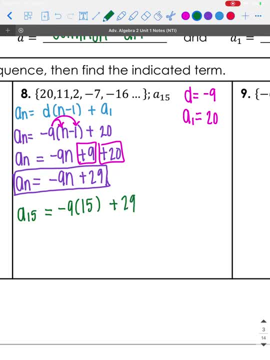 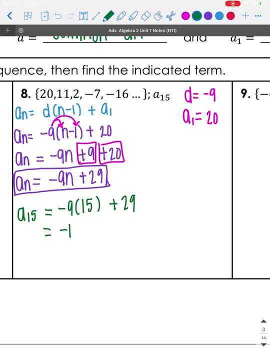 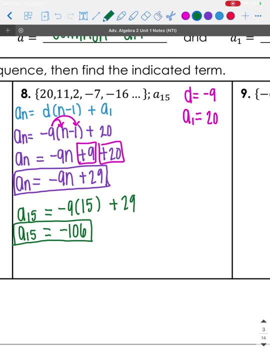 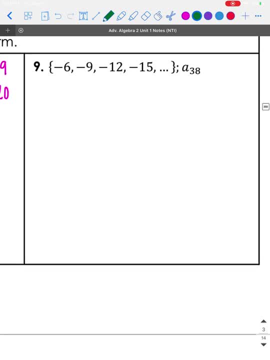 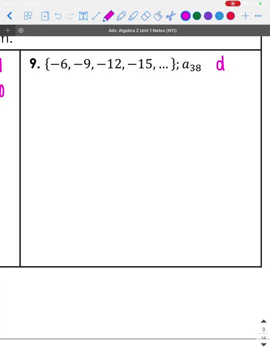 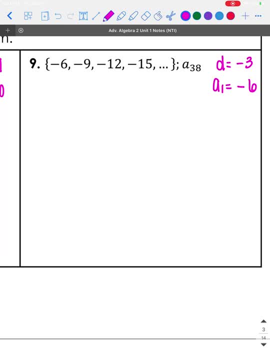 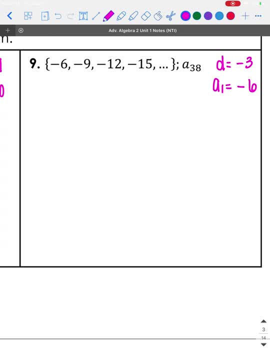 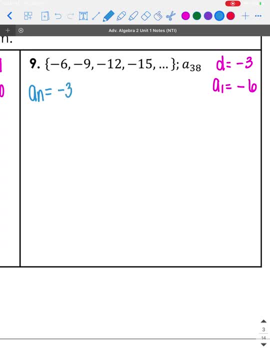 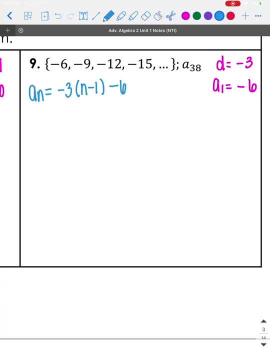 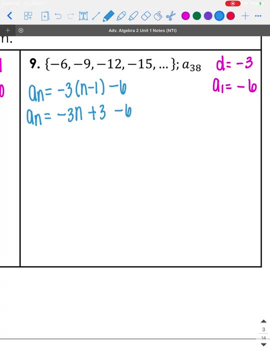 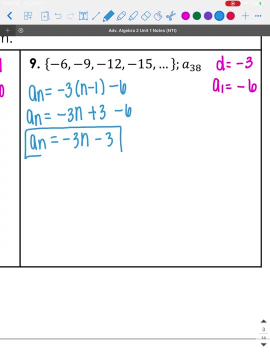 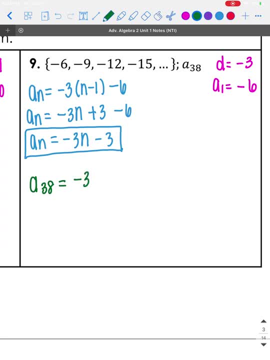 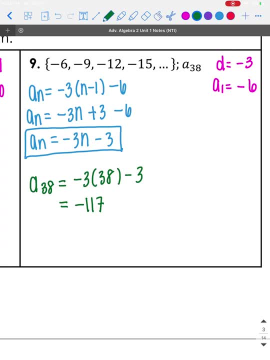 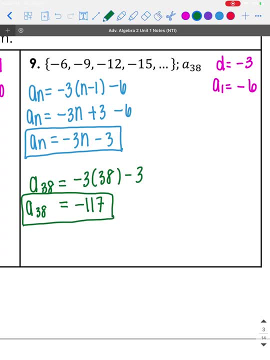 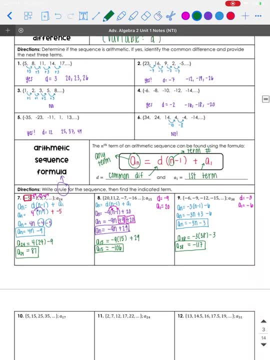 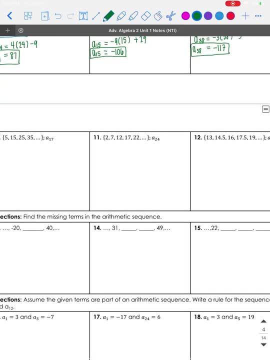 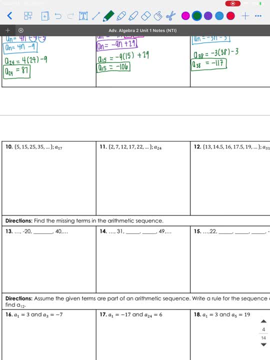 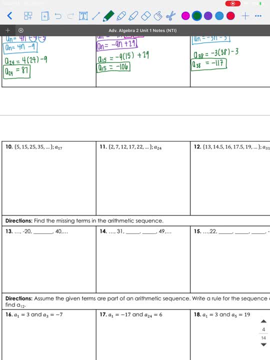 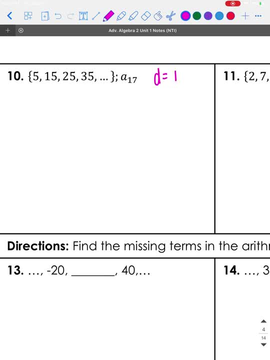 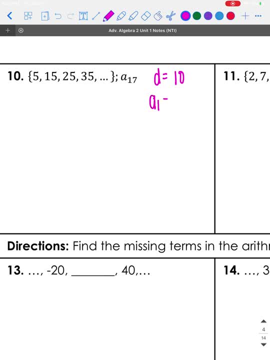 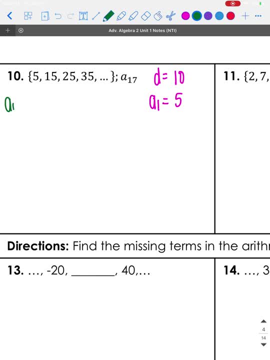 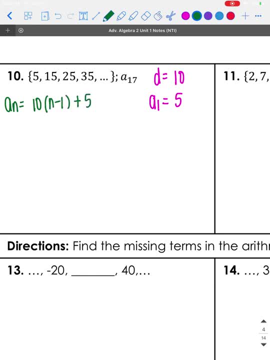 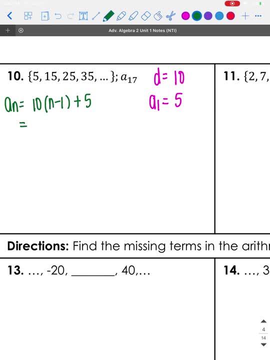 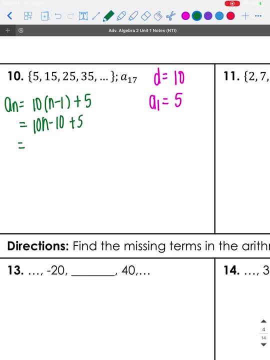 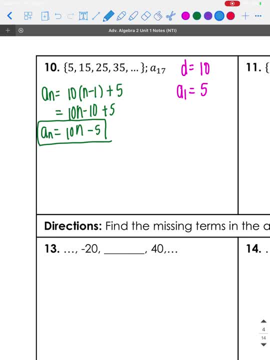 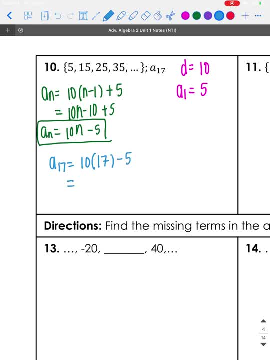 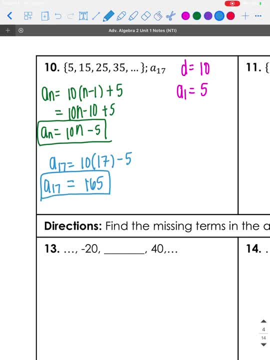 Distribute. Distribute. So your formula is A sub n equals 10n minus five, 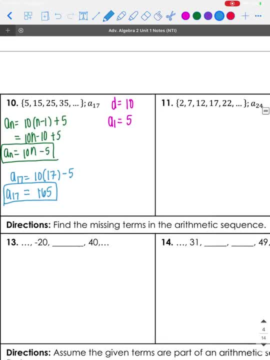 and the 17th term is 165. 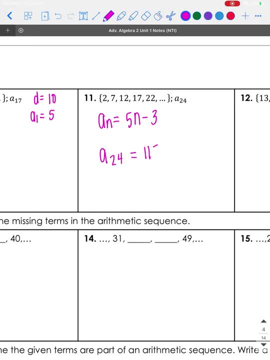 For number 11, your formula is a sub n equals 5n minus 3. 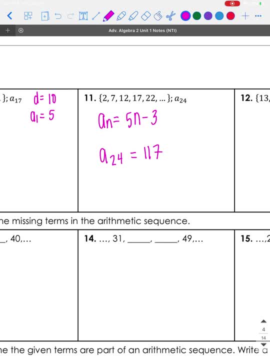 And the 24th term is 117. Number 12. 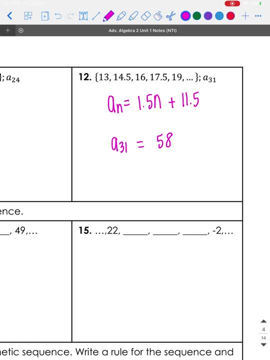 This one might have been a little tricky because it was increasing by a decimal, but any time you're calculating a decimal, you're confused and you don't know what the common difference is. 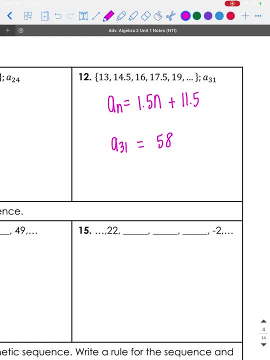 If you take any term, so let's say I take 17.5, you're going to subtract the one before it, minus 16, and you get 1.5. 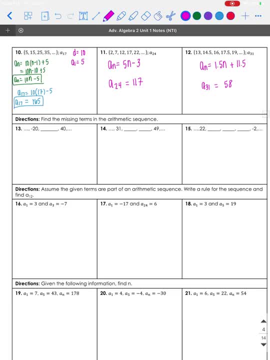 All right, we have just a few more types of questions. So let's look at number 13. 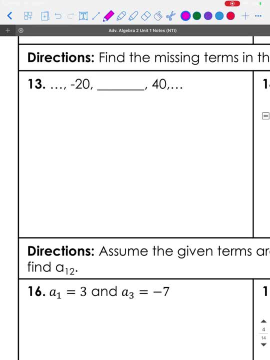 We are missing a term in the middle. So if you think about an arithmetic sequence, what happens in an arithmetic sequence? How do you get from term to term? What we do is we add some number that we call the common difference. Right? 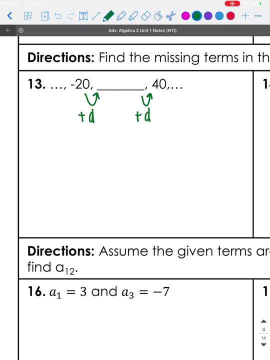 So if I were to go from negative 20 to that number, I would be adding whatever d is. And then I would go from that number to 40. I'm still adding that same number. So I'm going to set this up as an equation. I'm going to say if I go from negative 20, I'm going to do... 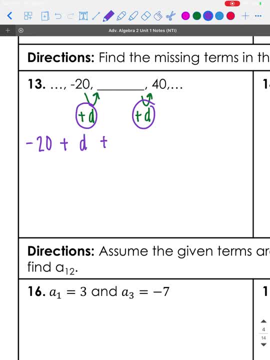 plus d. And then I plus d again to get 40. 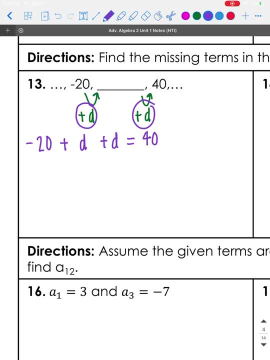 So I started at negative 20. I added that common difference twice to get to 40. 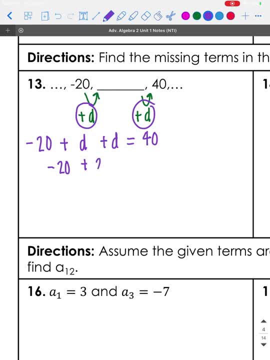 And I get negative 20 plus 2d. Plus 2d. Plus 2d equals 40. 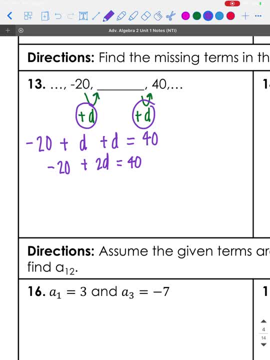 And then I just solve this like an equation to find my common difference. Add 20 to both sides. Then divide by 2. 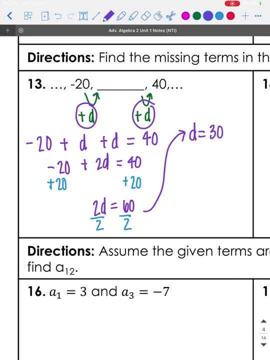 And we get that our common difference is 30. That does not mean that what goes in the blank is 30. That means that the common difference is 30. 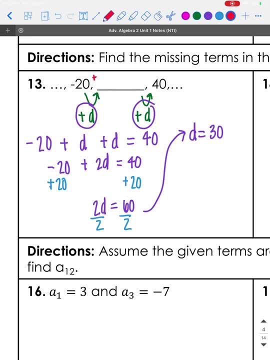 So to find what's in the blank, I'm going to take negative 20 plus 30. And that gives me 10. 10 goes in the blank. 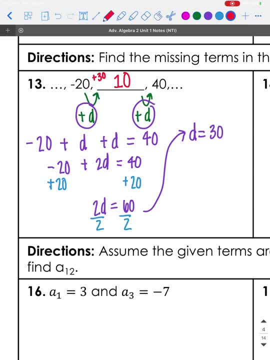 And if I did that again, 10 plus 30 is, in fact, 40. 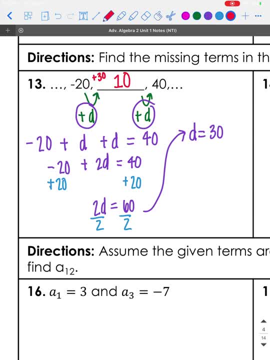 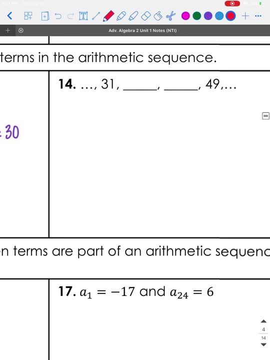 All right. Let's look at number 14. 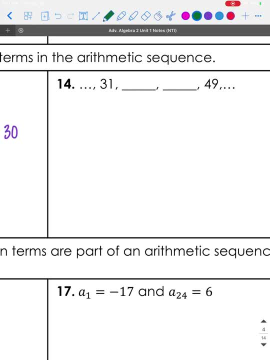 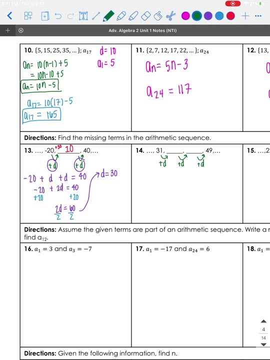 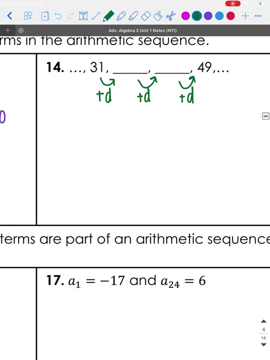 Same thing, except this time I have two blanks. So if I add my common difference... 10 plus 30 is... It's going to look very, very similar to number 30. Except this time I'm adding the common difference three times. So I'm going to have 31 plus 3d equals 49. And then if I solve that... Okay. 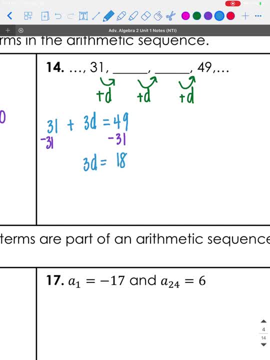 Subtract 31 from both sides, we get 3D equals 18. And then I'm going to divide both sides by 3. To get D equals 6. That means that my common difference is 6. I am adding 6 every time. So to find out what goes in the blank, 31 plus 6 is 37. 37 plus 6 is 43. And 43 plus 6 is 49. 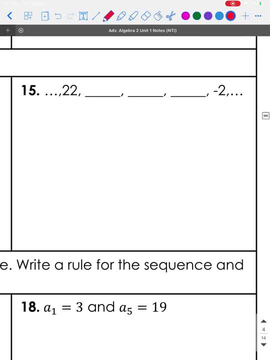 Try number 15 on your own. So pause the video. Work number 15 out to make sure that you understand. And then we'll move on. 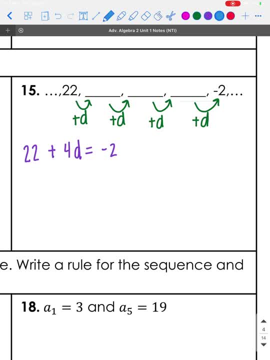 D equals negative 6. If you did not get that, look at your work compared to mine. Make sure that you have 4D instead of 3D or 2D. And make sure you solve correctly. And then so that means I'm subtracting 6 every time. 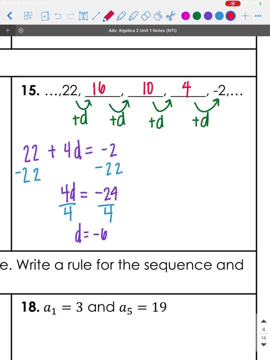 16, 10, and 4 go in the blank. 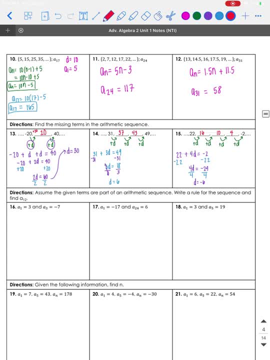 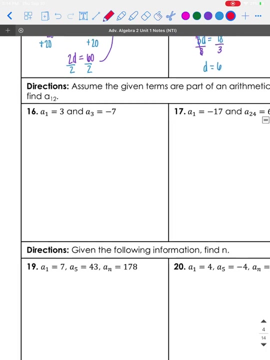 Alright, so what we just did in questions 13 through 15, we're finding... We had to find the common difference. And then from there, we filled those back in, right? So we use what's called arithmetic means. Now, I didn't really tell you that was arithmetic means, but we round about did that. 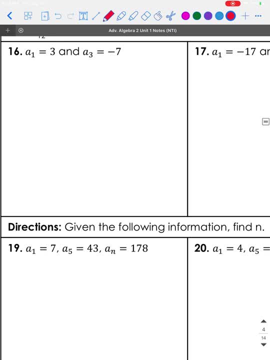 So I'm going to show you another way to find the common difference in examples like these. Where you don't actually see the blanks. I'm just giving you the example. So I'm going to show you another way to find the common difference in examples like these, where you don't actually see the blanks. I'm just giving you two terms. 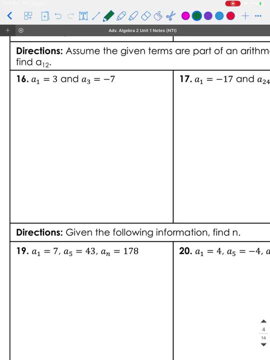 So in order to do that, we're going to look at these two terms. 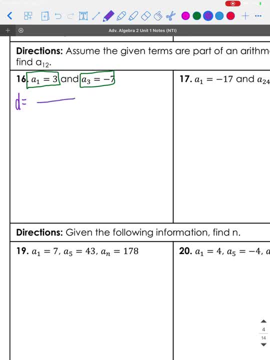 On the top, I'm going to make a fraction. So my common difference, I'm going to make a fraction. 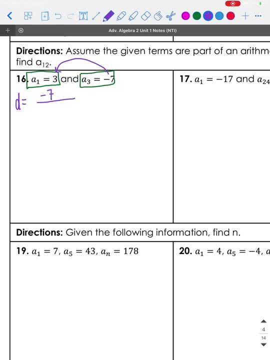 On the top, I'm going to take negative 7 minus 3. And on the bottom, I'm going to take 3 minus 1. 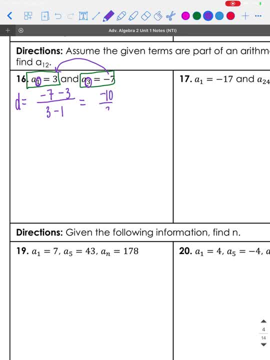 And that gives me my common difference of negative 5. 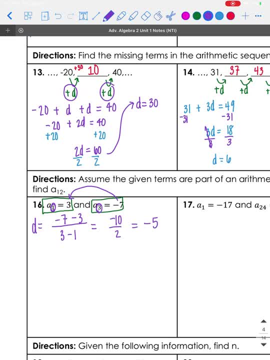 That would have worked up here if I would have, for like number 13, if I would have said, okay, well, negative 20 is a 1, and 40 is a 3. That would have worked. 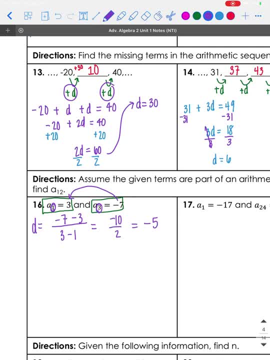 40 minus negative 20 over 3 minus 1, which is 2. That's kind of what we did, but in a different way. 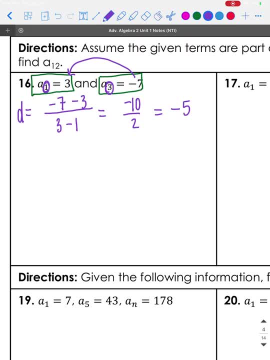 So this way that I'm showing you in number 16 works just as good or better, I think. 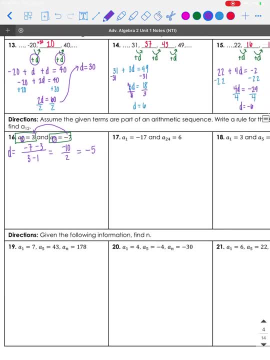 So this question says, we didn't even really answer the question. Assume the given terms are part of an arithmetic sequence. 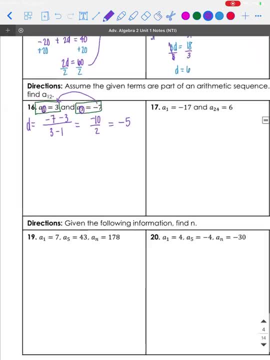 Okay. Write a rule for the sequence and find a sub 12. So in order to write a rule, I had to have that common difference. So we're good. 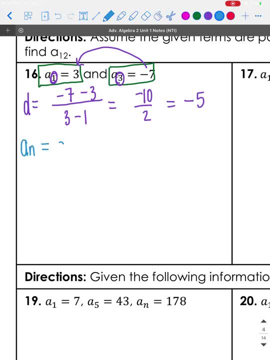 So remember your rule, or your formula, is your d times n minus 1 plus a1. I just found this. Okay. just found my difference was negative five. My A1 is three. Distribute. I distributed 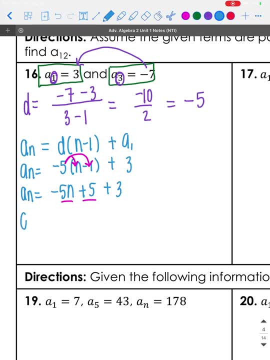 there. Combine your like terms. That is your rule. A sub 12. I'm just going to plug 12 in. 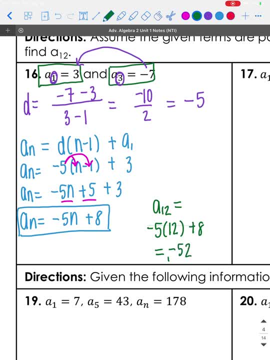 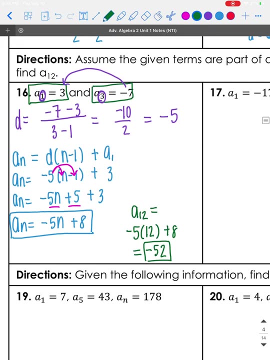 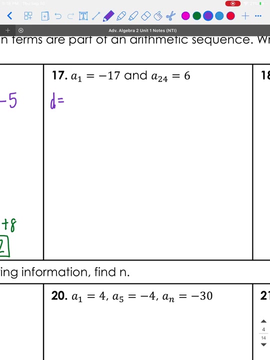 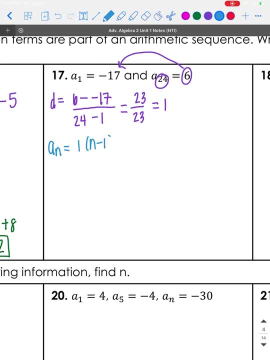 Or write the formula. So my common difference is one times the quantity n minus one plus my first term, which is negative 17. If I distribute one times n is n. One times negative one is negative one. 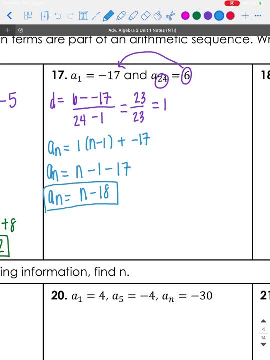 So my rule is n minus 18. 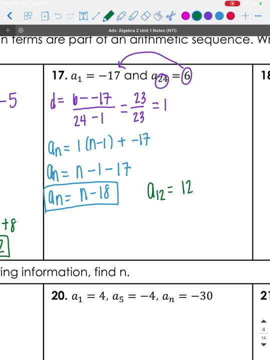 And then I need to find A sub 12. 12 minus 18 is negative 12. So now I'm going to take both of my problems. I grad them. One times n minus 12 is negative 1. I'm going to take both of my problems. 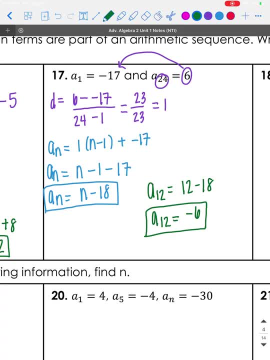 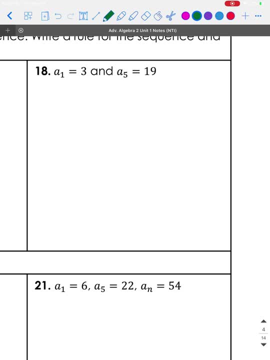 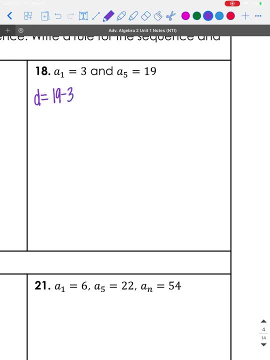 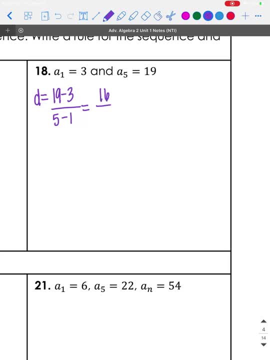 Thank you. All right, for number 18, you should get that the explicit formula, or the rule, is 4n minus 1, and for the 12th term, we get 47. 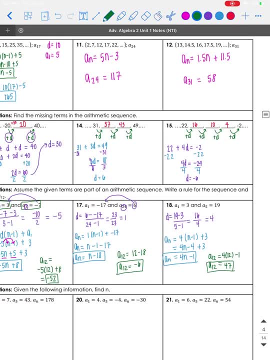 All right, we are almost done. I am so sorry that this has lasted so long. 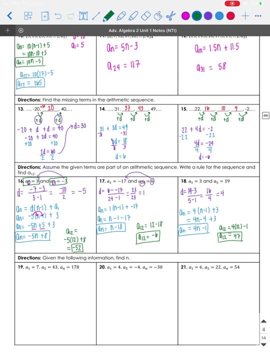 Hopefully, you've paused it, took a break, if you needed to, came back to it later. 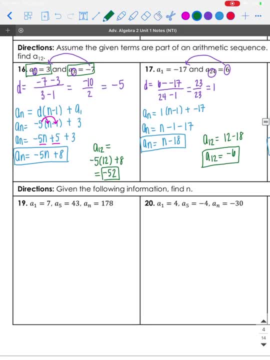 But the last three questions that we have are similar to the 16, 17, and 18. So, let's look here. 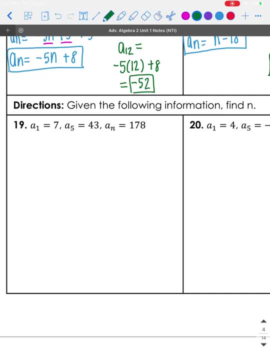 Given the following information, find n. So, right off, something that's new is this. a sub n equals 178. That's new. 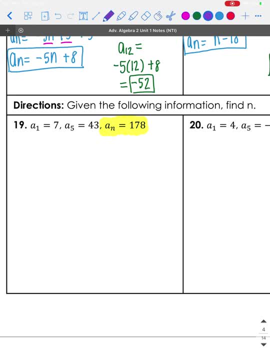 I still notice that I don't know my common difference, and that's something you know how to find. 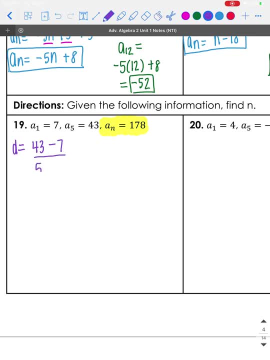 43 minus 7 over 5 minus 1. 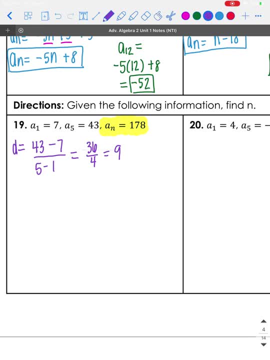 So, that's something, if you don't know right off, figure something out. See what you know how to find, and maybe it'll hit you how to do it. 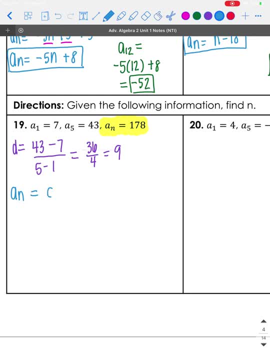 If I think about my explicit formula, looking at what the problem gives me, does it tell me what an is? Yes, a n is 178. 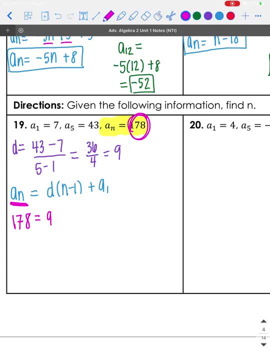 Do I know what the common difference is? Yes, I just found it. 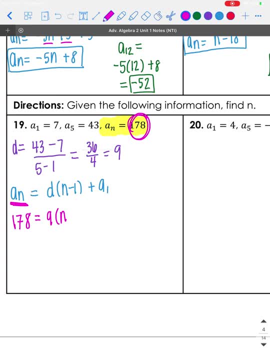 Do I know what n is? No, the problem is asking me to find it. 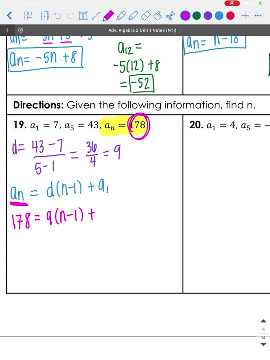 Do I know what a 1 is? Yes, it is 7. 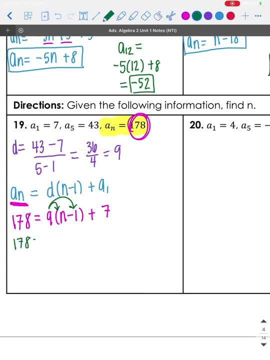 I can now distribute, combine like terms, and I can actually solve this. If I add 2 to both sides, combine like terms, combine like terms, then I can actually solve this. 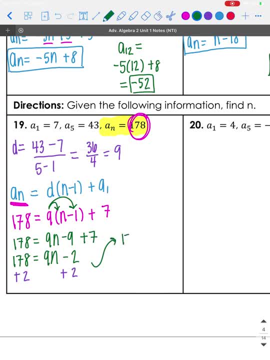 If I add 2 to both sides, and I'll leave n prime, I'll get n prime. This way, I can actually solve this. 178 plus, oops, 178 plus 2 is 180, equals 9n. And then I can divide both sides by 9 to get 20 equals n. 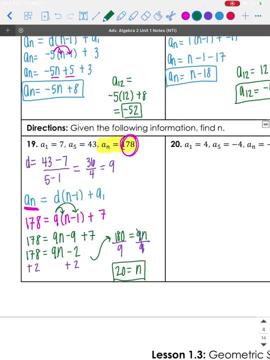 So my n is 20. And all of these problems, if you look at it and you're like, oh my goodness, I have no idea. Start somewhere. 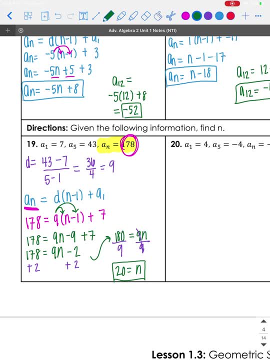 See what you can figure out. Look back at the formula. See what you can plug in. It may get you one step, and then every time you get a new step ahead, you may realize something or be able to do something else. 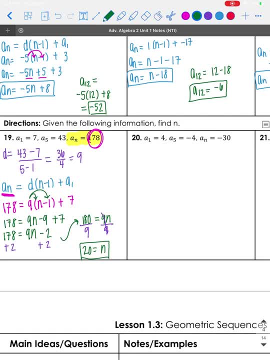 So number 20, same pattern. I'm going to start by finding my commonality. Common difference. Common difference is negative 2. 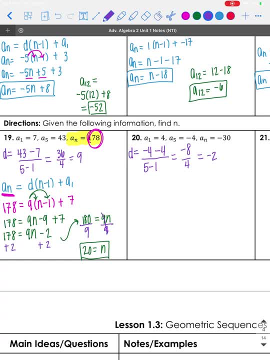 And then plug what you know into the formula. I know. That. 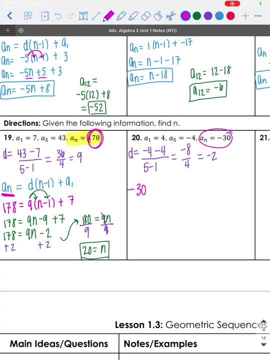 A sub n is negative 30, because the problem gives me that. I know that the common difference is negative 2, because I just figured that out. I don't know n, so I have to leave it. But I do know that my first term is 4, because the problem also gives me that. Okay. Now we can distribute. Combine like terms. And then solve. 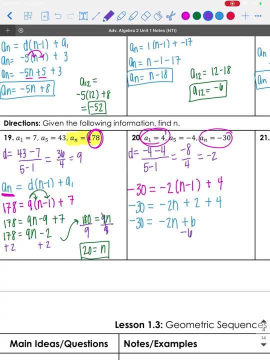 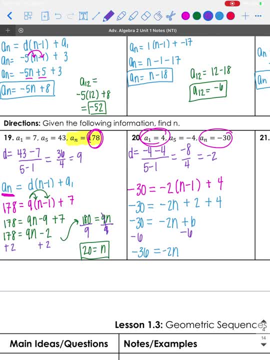 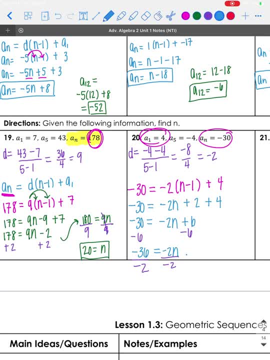 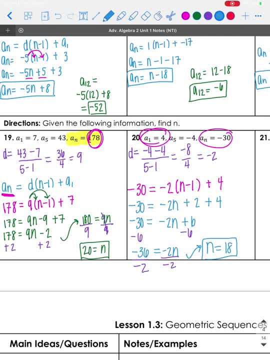 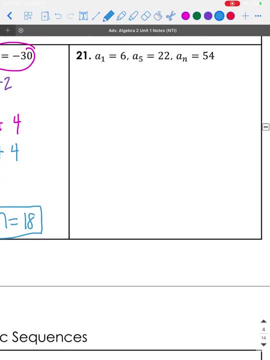 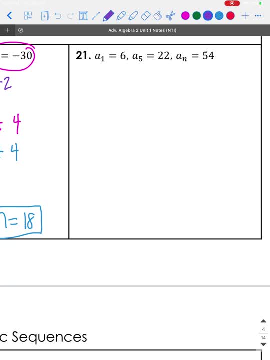 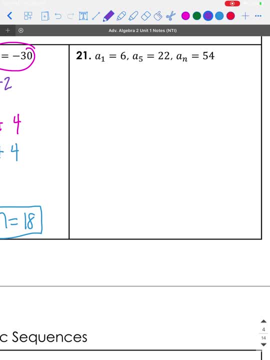 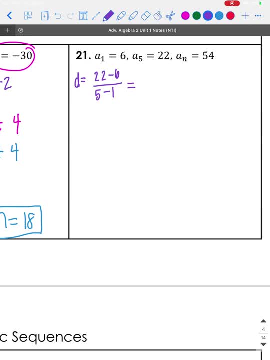 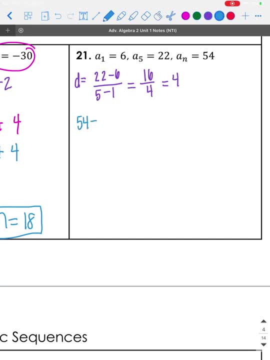 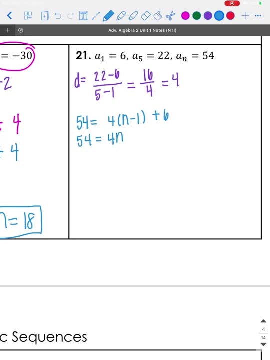 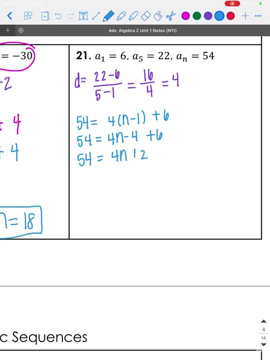 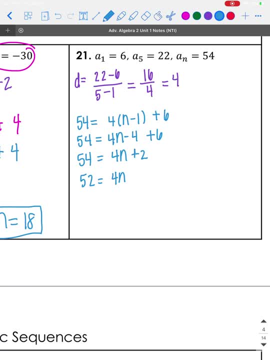 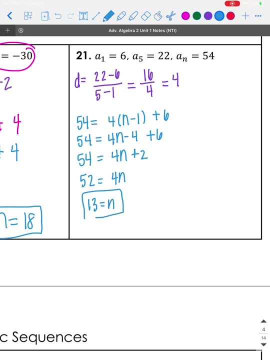 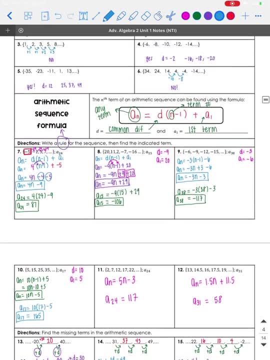